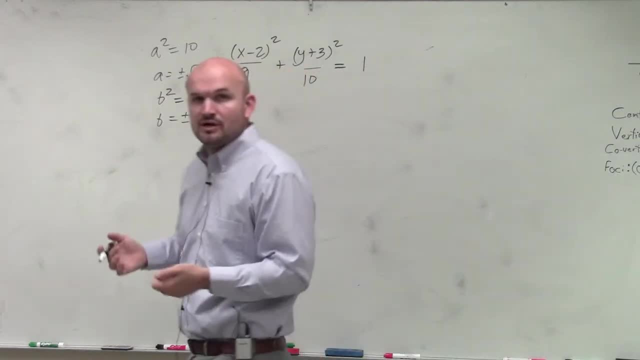 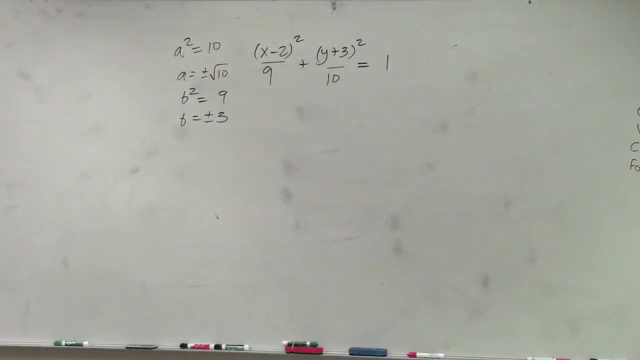 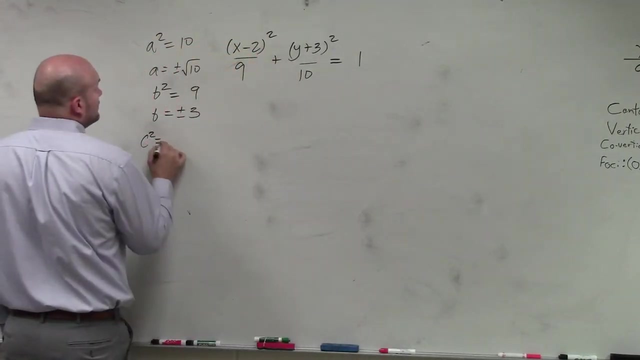 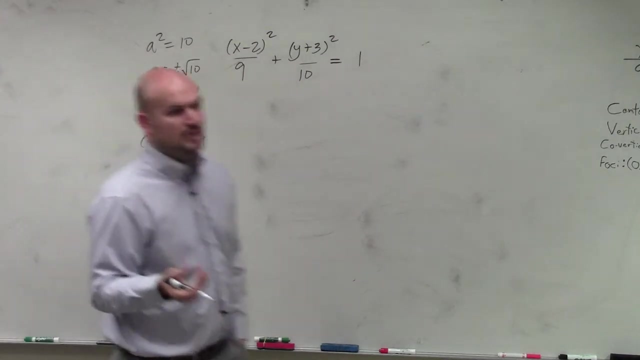 well, I know I'm going to have to find c. anyways, you could go ahead and find your c. So c squared would equal 10 minus 9.. c equals plus or minus 1, right, Correct, OK, All right. 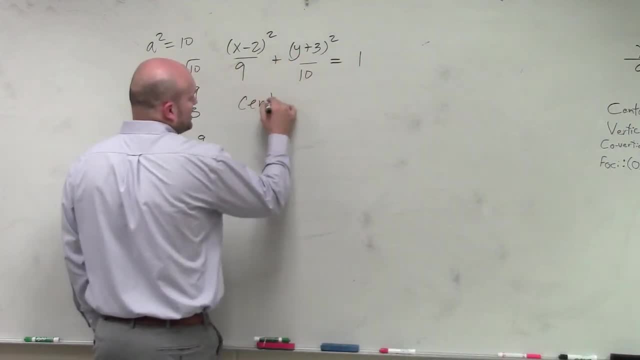 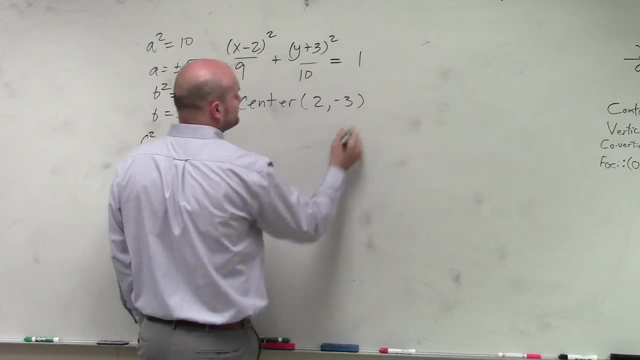 So let's go and find the center. The center is going to be your h comma k, So remember it's x minus h, y minus k. So therefore your center is 2 comma negative 3.. So we'll go ahead and plot that information. 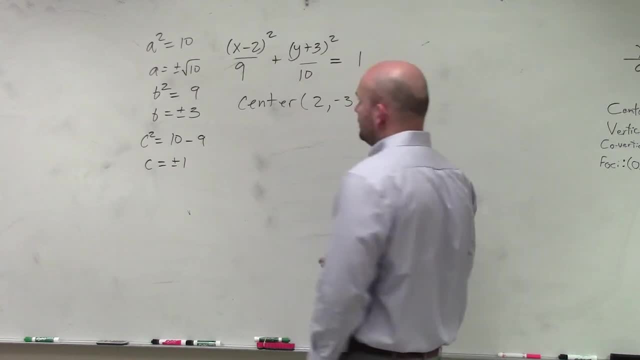 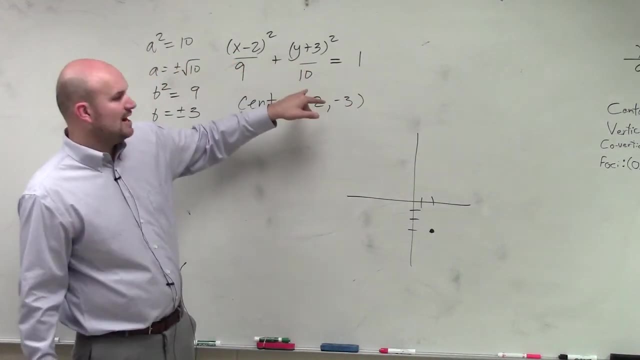 1, 2, 1, 2, 3.. OK, Now again we need to identify our major axis. Is it vertical or is it horizontal? Well, since my a squared is under my y, that means I have a vertical major axis. 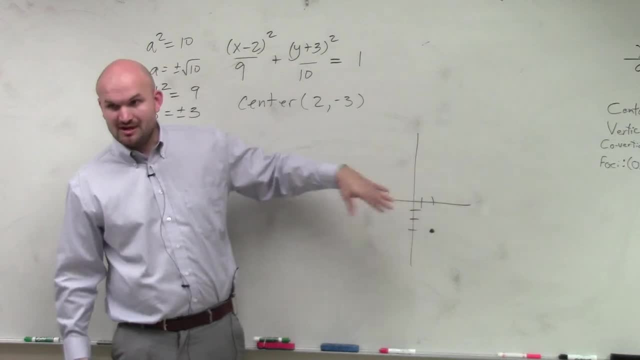 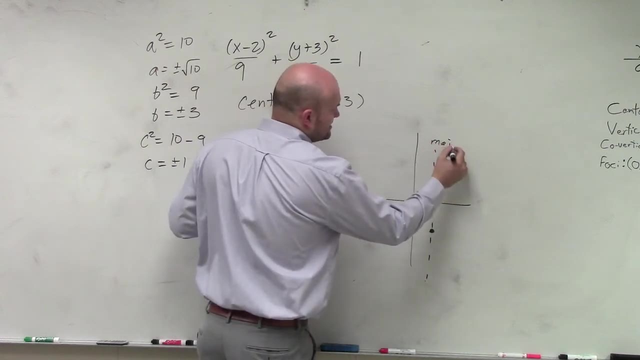 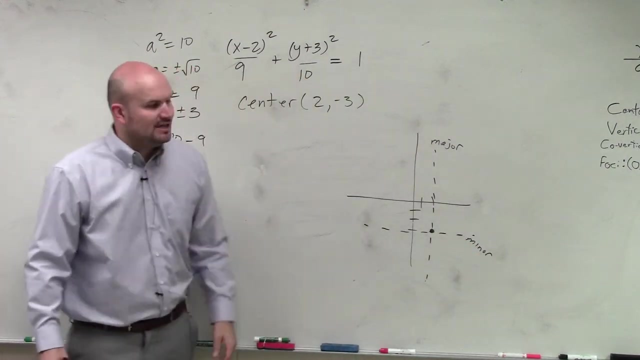 Now, Since my center is not on the origin anymore, I am going to put a major axis there. You don't have to do this, but I have found out in my experience that actually writing the major axis and the minor axis helps people avoid making mistakes. 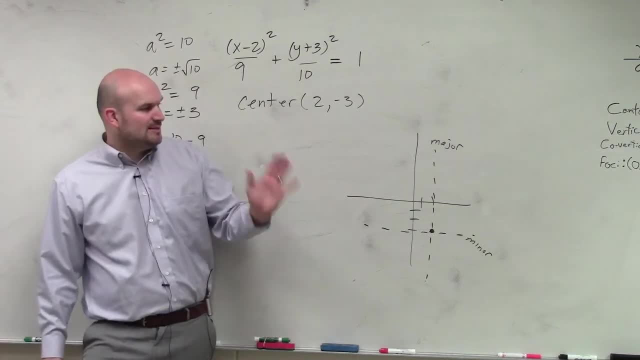 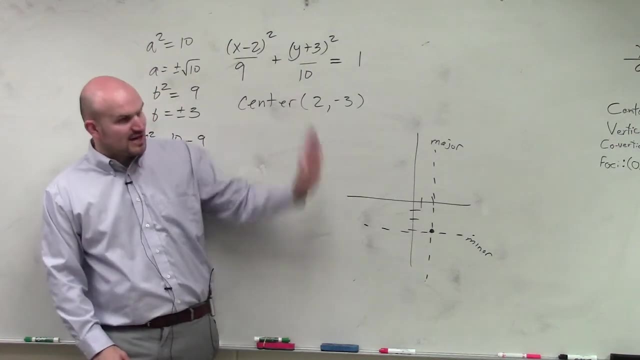 Because what do people do? They forget. They forget where the major axis was. They put the foci on the minor axis, Whatever. So I always just like to write. I just put little dash lines there saying, hey, here's my major axis. 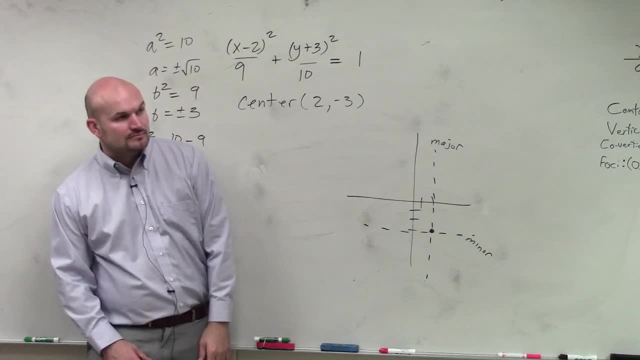 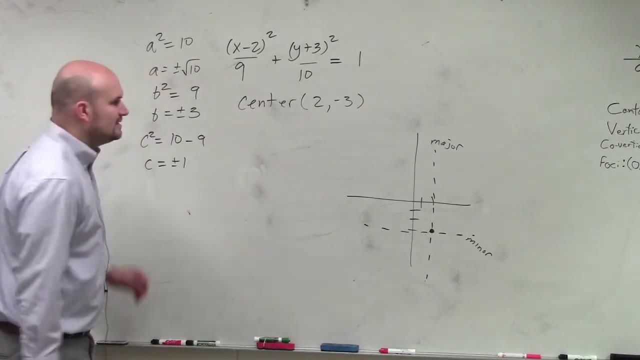 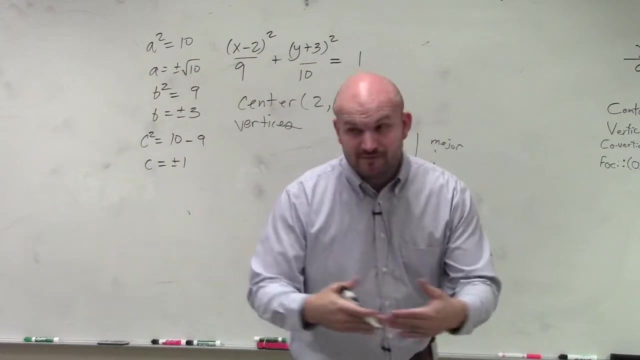 There's my minor axis. Yes, So is the major axis always going through the center. Major and minor always intersect at the center. So the next thing is to find my vertices. So the vertices, remember, is a distance a away from the center. 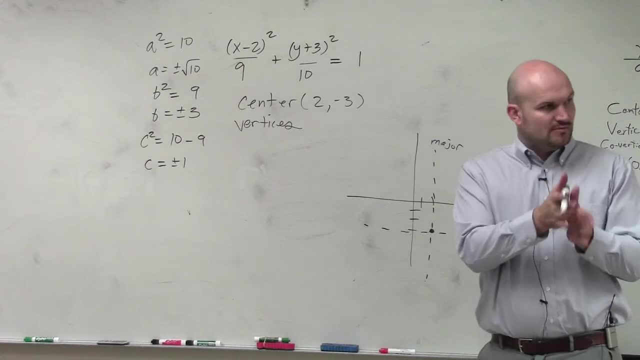 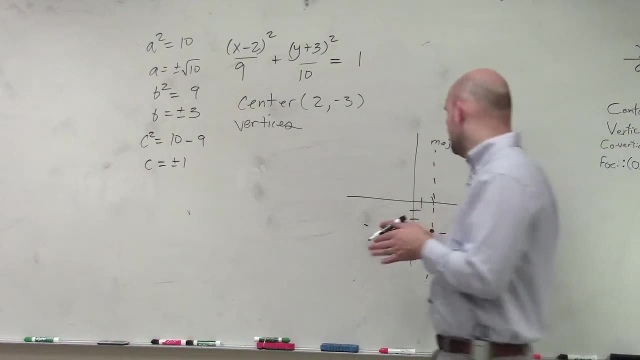 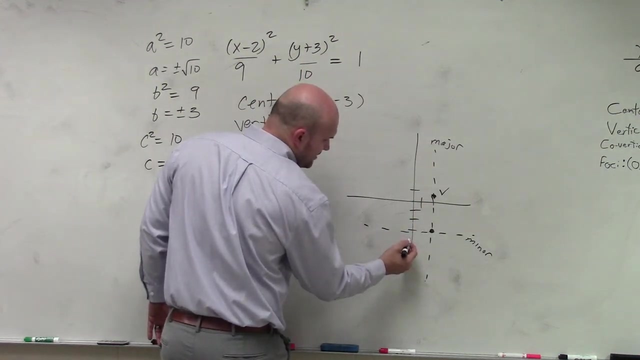 And that distance a is square root of 10, which is roughly somewhere between 3 and 4.. So I'll just go up 3.. 1,, 2,, 3,, 4.. So that's somewhere right there, And then go down 3 and add somewhere. 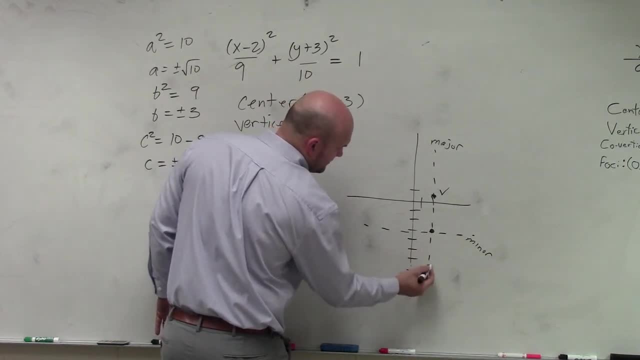 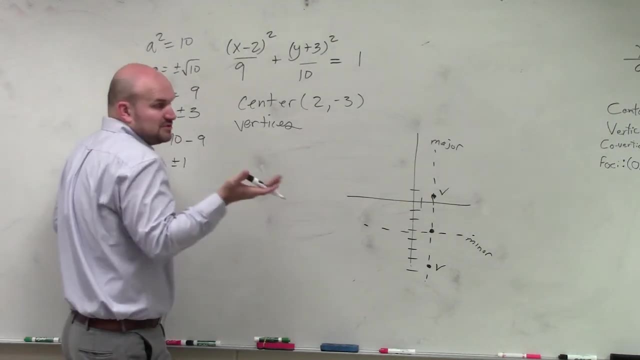 1,, 2,, 3, 4.. So somewhere right there- Wait, No, that's square root of 10.. Yeah, Square root of 10 is what Between 3 and 4, right, So let's write these in there though. 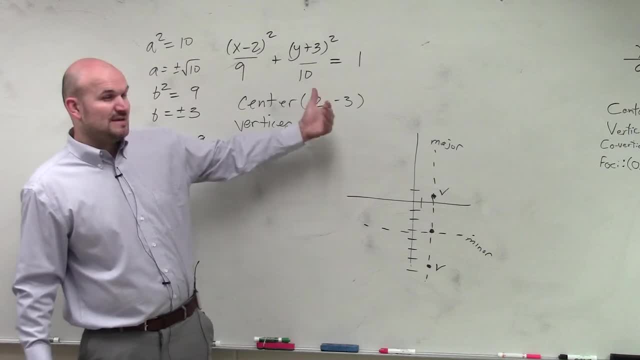 So you guys can notice that I'm going up and down. So therefore, should I be adding and subtracting 10 to the square root of 10, to negative 3? Or should 2?? Well, if you're adding and subtracting to 2, that's going. 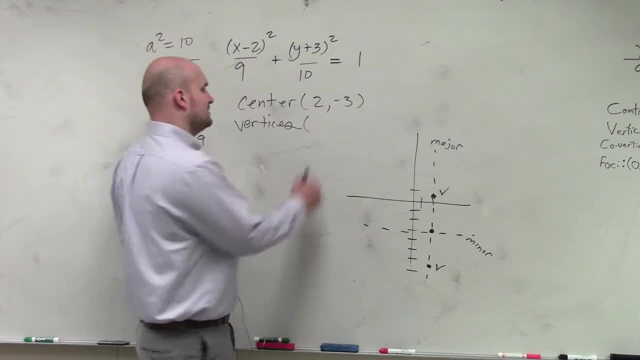 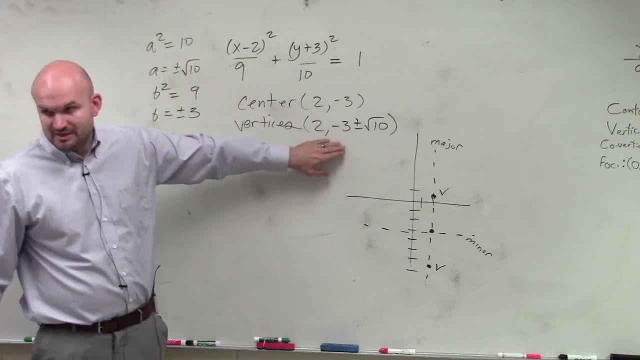 to move. It's going to move it left and right, So we've got to go up and down, So that's to negative 3.. So I do 2 comma negative 3, plus or minus the square root of 10.. I'd prefer if you guys would leave it in that format. 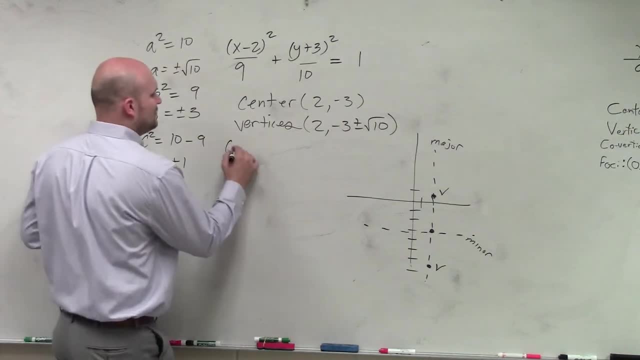 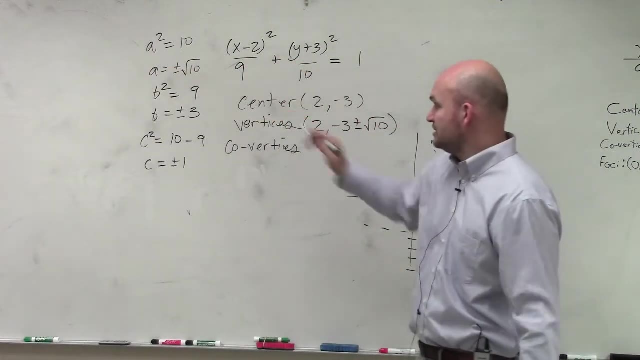 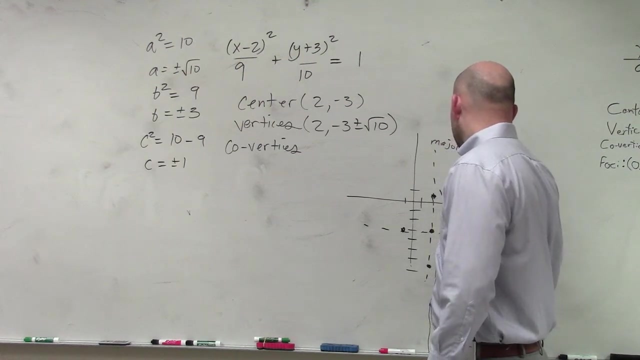 You can separate it, but that is perfectly fine. The co-vertices are going on the minor axis, a distance of b, which is in this case 3.. So 1, 2, 3. And 1, 2, 3.. 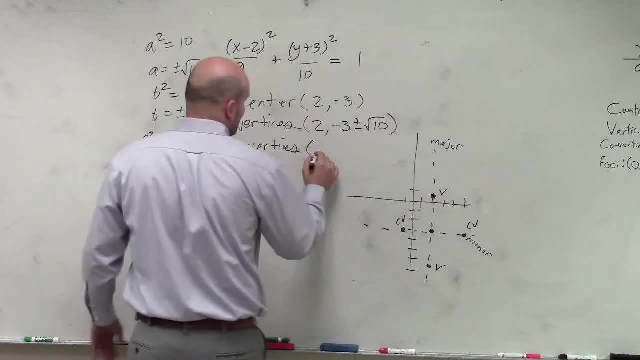 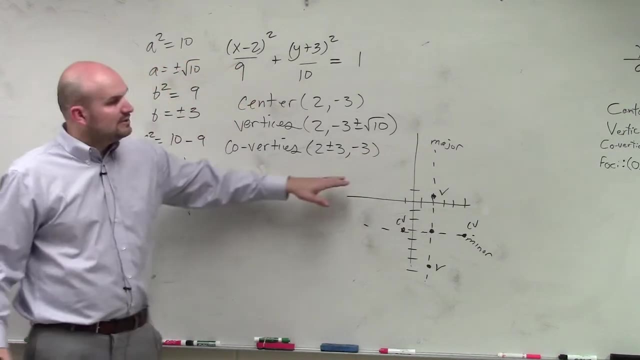 Co-vertices, co-vertices Which in reality really what I'm doing is. I'm doing 2 plus or minus 3 comma negative 3.. Now, I would prefer that you not leave your answer like this. To me that's kind of lazy. 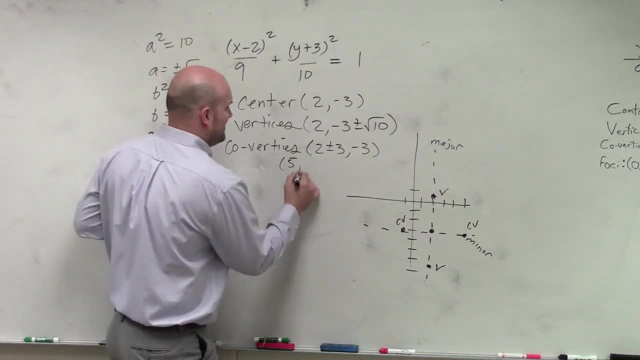 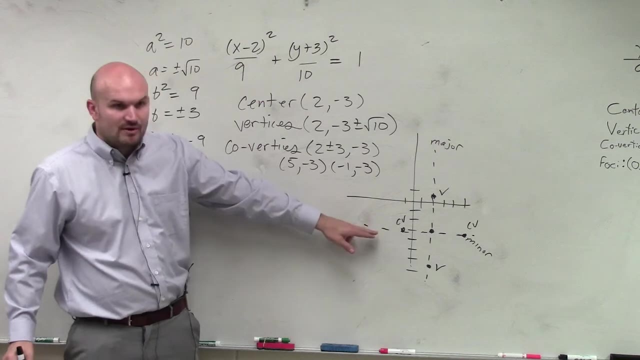 We can easily add 2 plus 3, right, That's 5 comma negative 3.. And then 2 minus 3 is negative, 1 comma negative 3.. And guys do those points. look about right from where we plotted them. 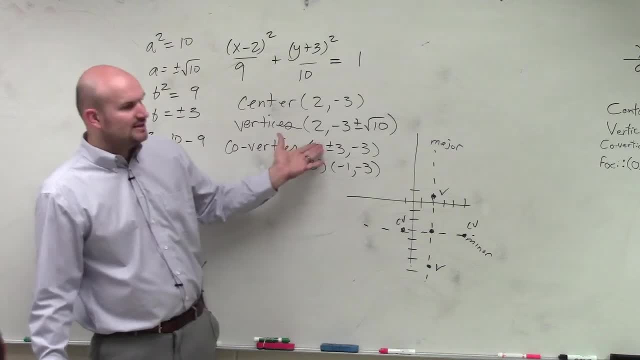 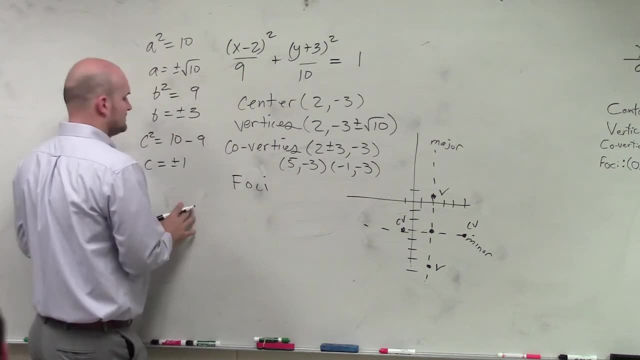 No, Well, right, right. So you don't even have to write the formula things, You could just go by your graph if you wanted to. And then, last but not least, is the foci. Foci is plus or minus 1.. 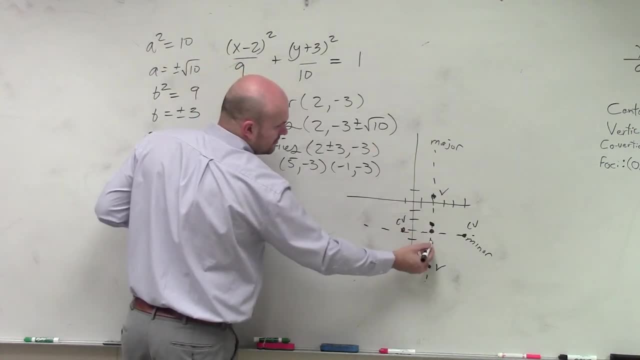 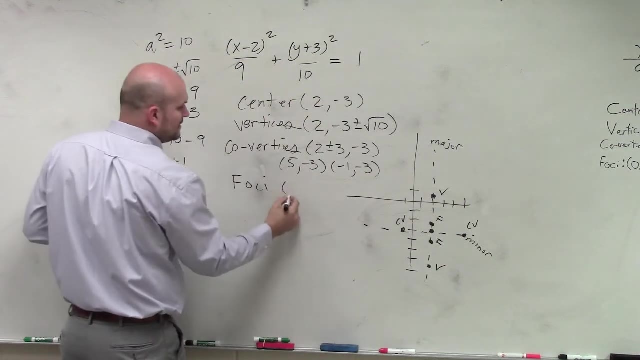 But remember, it's on the major axis. So there's your foci. There's your foci. That's going to be plus up and down from negative 3.. So that's going to be 2 comma negative 3 plus or minus 1.. 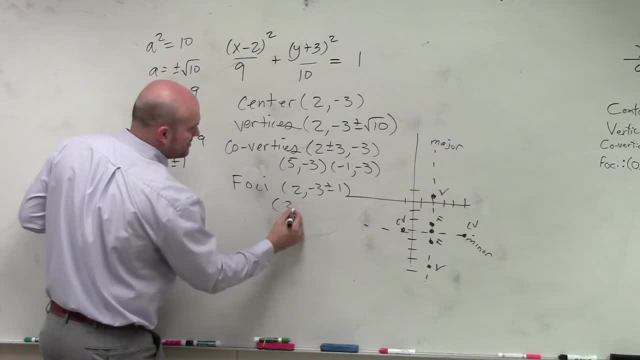 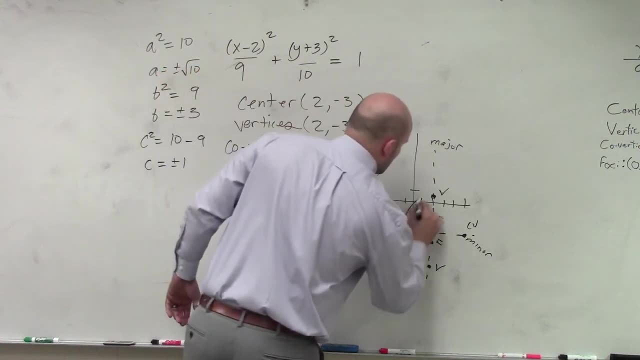 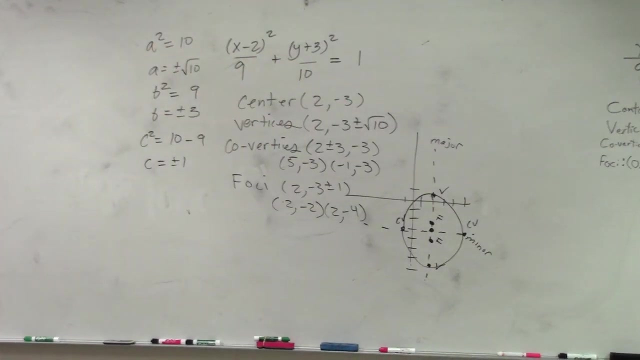 Which is, again. I'm only writing this out so you guys can see where my math is coming from. Let's see That's going to be 2 negative 2 and 2 comma negative 4.. So I have two problems that are up there on the board.